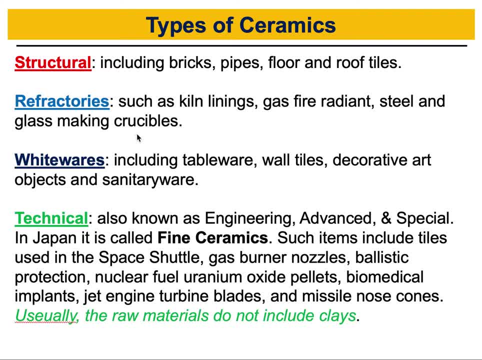 pieces of equipment that withstand a lot of heat. That's why we use ceramics there. Also, we have something called the whitewares, including the tableware, wall tiles, decorative art objects, So we are also familiar with that. Now these days. we developed something called technical ceramics. 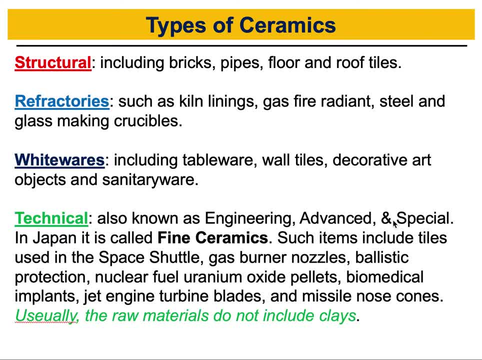 and also known as engineering, advanced or special ceramics- In Japan they call them fine ceramics- and such items include high-end applications, pieces of equipment or parts that for a very advanced- you know- applications, So they're used in space shuttles, ballistic. 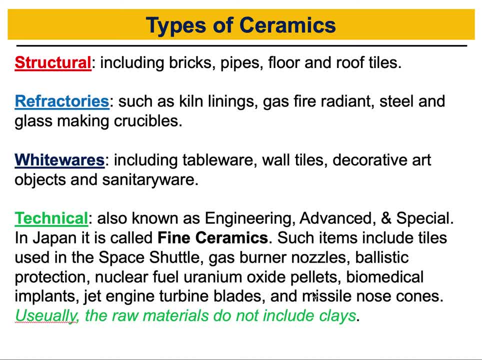 protection, nuclear fuel, uranium oxide pellets, a lot of biomedical materials, implants for biomedical applications, jet engines. So there's a wide range of applications. when we call it technical- Sorry, there was a typo here- It's usually, and usually the raw material do not. 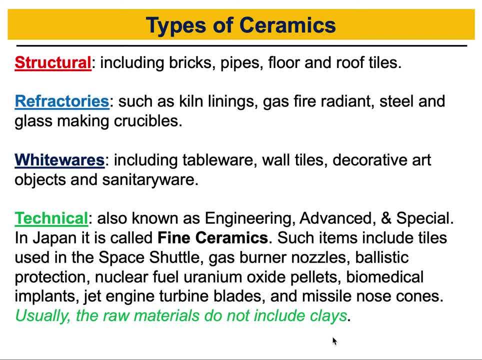 include clay. Clay is when we term the ceramics as technical ceramics or fine ceramics. So those are the four types that are characterized by application of ceramics. We need to learn more about ceramics, We need to look into them. What are the internal structure of the ceramics, How are they made and what are the elements that make ceramics? 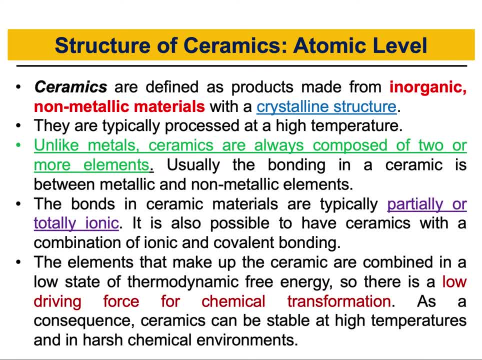 So if we look at the structure of ceramics and we went to the atomic level, So ceramics are defined as products made of inorganic, non-metallic materials. So they're not metals and not organic. and when we say organic, there's organic means materials that are bound inside biological tissue: carbon. 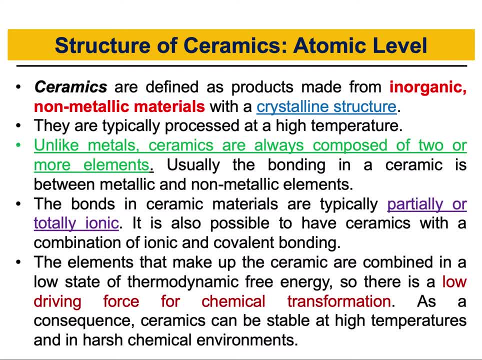 hydrogen oxygen. Those are organic materials. Inorganic are the other materials and also there should be non-metallic. Interestingly, they have crystalline structure. Sometimes they don't have crystalline structures, but most times they have crystalline structures Also. so we want to keep these in mind when we study or think about ceramics. So inorganic material. 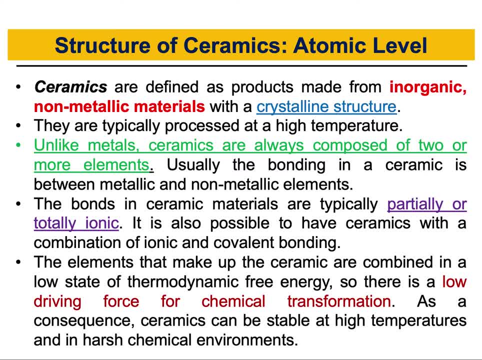 elements. they are non-metallic and also they they have crystalline structures. Also they're typically processed at high temperature, So because they withstand a lot of temperature. Unlike metals, ceramics are always composed of two or more elements. So we can't find ceramics made of a pure one element, one element purely.